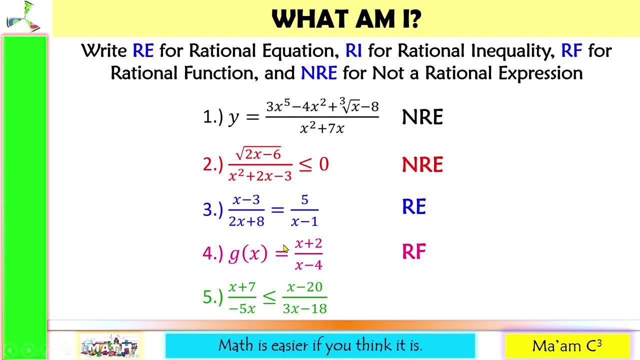 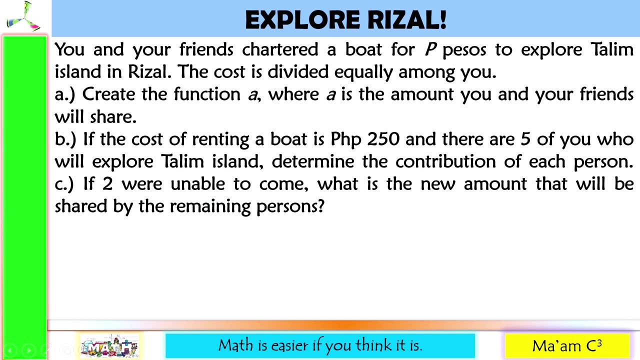 We have here the name of the function and the equal sign. And last one, this is NRE, because of the square root here. Number three: this is a rational, is a rational inequality. both sides are rational expressions with inequality symbol in between. let us explore result: you and your friends chartered a boat for p pesos to explore talim. 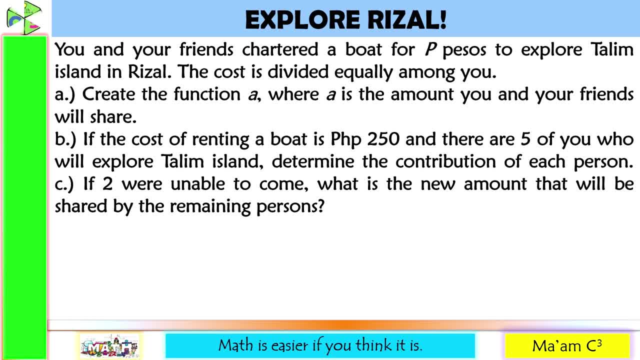 island. in result, the cost is divided equally among you. letter a. create the function a, where a is the amount you and your friends will share. so we're going to create a function- let's label it as a- and it is dependent on the number of friends who will share the amount. so i will use a of f, the. 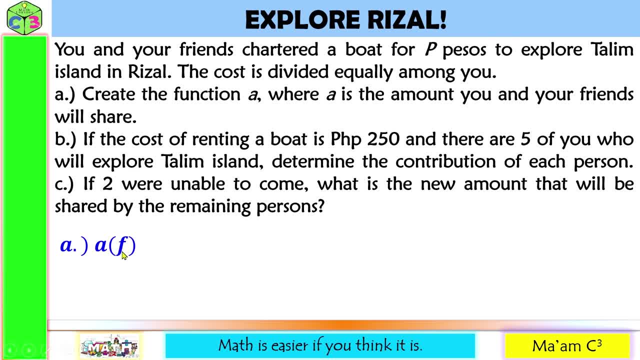 function name is a and it is dependent on the number of friends. so i choose letter f. so this is equal to the p pesos that will be divided by the number of friends. so p divided by f. letter b: if the cost of renting a boat is 250, 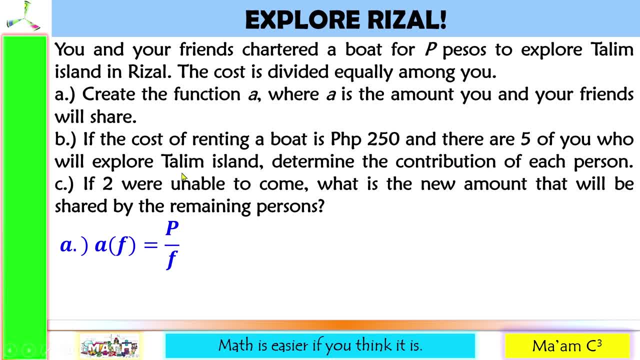 pesos and there are five of you who will explore talim island. determine the contribution of each person. so there are five persons who will share the contribution. so f here will become five, a of five, and then the cost of renting a boat is 250, so this will be a of five. is equal to 250 divided by 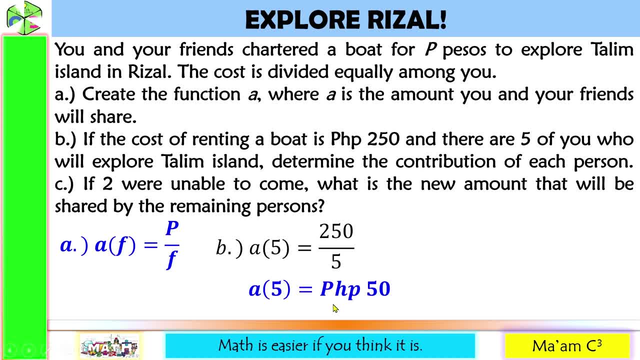 five, and this is the amount which is going to be divided by five. so p will be divided by five and equal to 50 pesos. So each one of you will contribute 50 pesos. Let us see, if two were unable to come, What is the new amount that will be shared by the remaining persons. So this time, 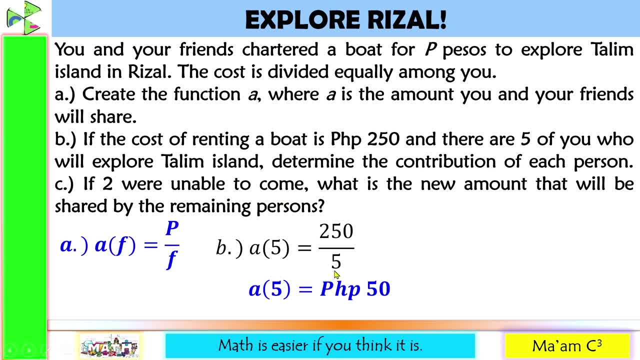 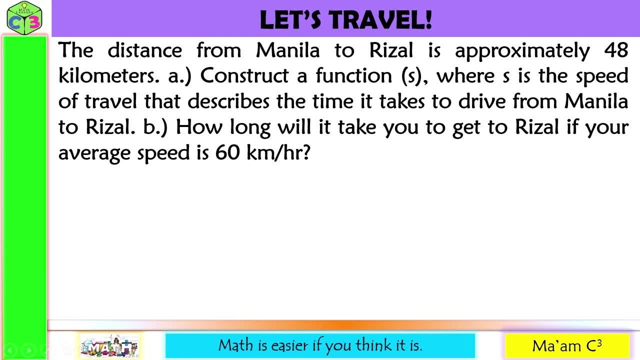 the friends that will share. the amount is no longer five but three, because two were unable to come, And 250 divided by three is equal to 83.33 pesos. Let us travel. The distance from Manila to Rizal is approximately 48 kilometers. Letter A, construct, a function S, where S is the speed. 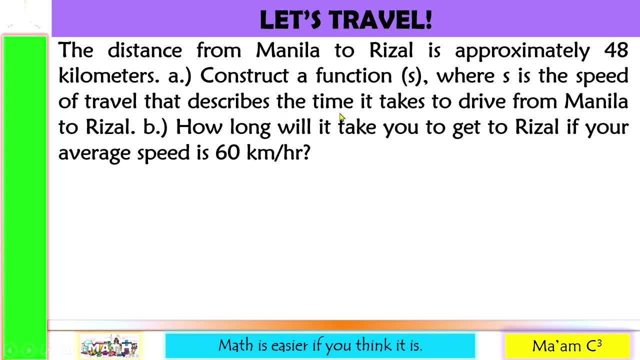 of travel. that describes the time it takes to drive from Manila to Rizal. Letter B: how long will it take you to get to Rizal? Average speed is 60 kilometers per hour. First, let me introduce to you the magic triangle. 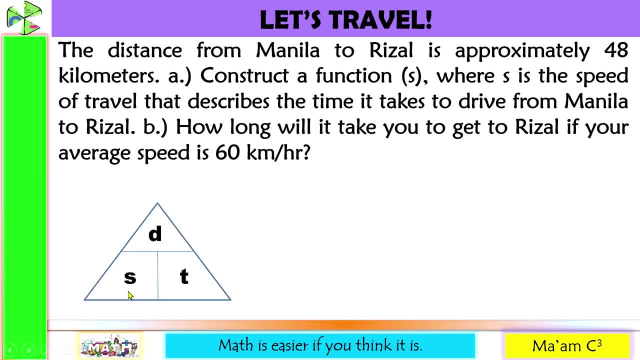 D here is for distance, S is for the speed and T is for the time. If you want to solve for the distance cover, the D. So D is equal to S times T. Now, if you want to solve for the speed cover, S. 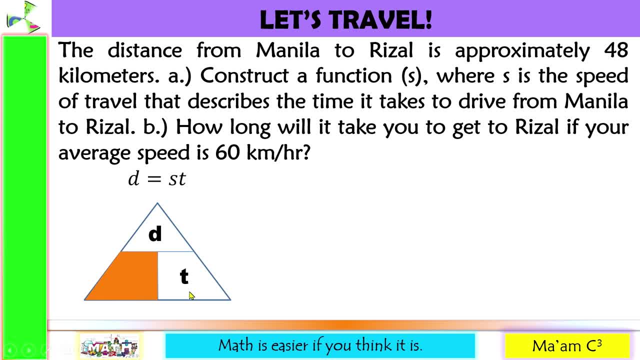 and S is equal to D divided by T. If you want to solve for the time cover, T and T is equal to D over S. Let's go back to letter A, construct a function S, where S is the speed of travel that describes the time, So function S. 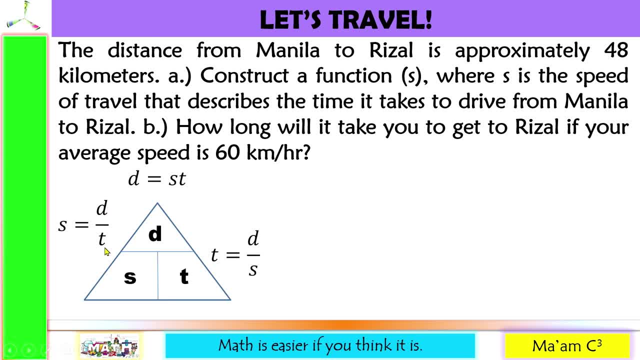 we're going to use this formula. S is equal to D over T, but the speed is dependent on the time, So S of T is equal to D over T. Letter B: how long will it take you to get to Rizal if your average speed is 60 kilometers per hour? 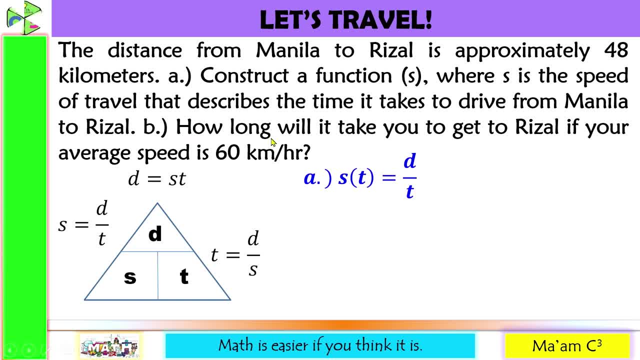 So this time we are asked of time- how long? So we're going to use this and the time is dependent on the speed. So our function will be: T of S is equal to D over S. The time is dependent on the speed. 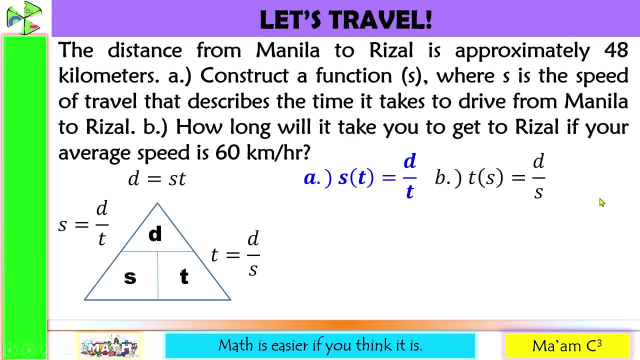 that whatever is your variable here, your right side of the function should also contain that variable. We have here t, So here we also have t. It says here: the speed is 60 kilometers per hour, So our s here is 60. So this will be: t of 60 is equal to d is given, and that is 48 kilometers. 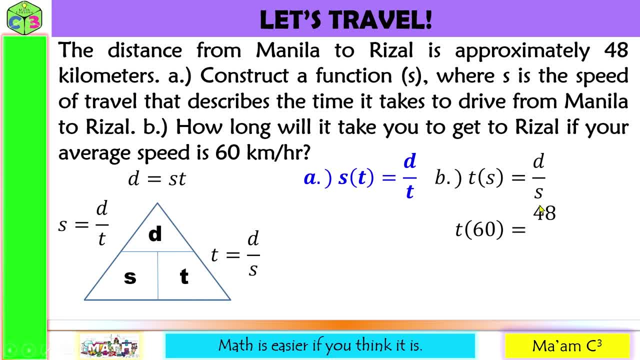 So 48 divided by s, again s, is equal to 60- the speed. and 48 divided by 60 is 0.8 hour, not even a one hour. To give you an idea, let us convert 0.8 hour to minutes: 0.8 hour times 60 minutes. 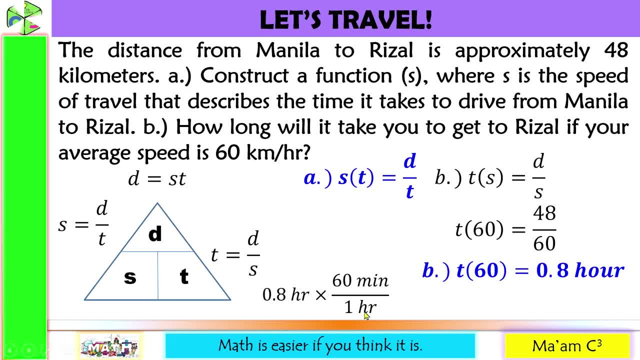 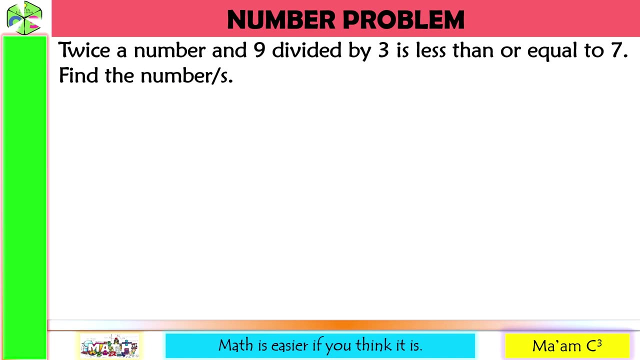 divided by one hour. So this hour here will cancel out 0.8 times 60.. 60 is equal to 48.. So 48 minutes, not even one hour. So what are you waiting for? Come on, let us travel to resolve Next twice a number and 9 divided by 3 is less than or equal to 7.. 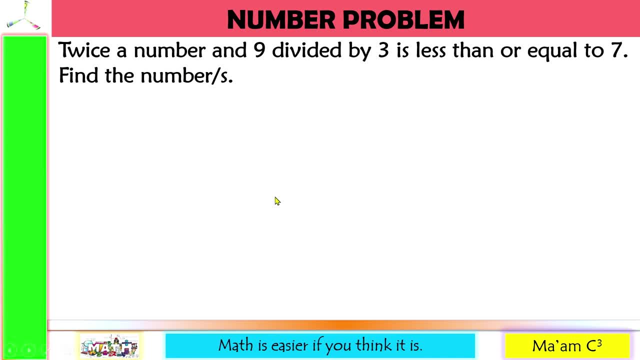 Find the number or numbers. Let's create an equation here: Twice a number and 9.. So that would be 2x plus 9.. Twice a number, we do not know. So let's create an equation here. We do not know the number, so we'll label it with x And 9, so we have plus 9. Divided by 3.. So all. 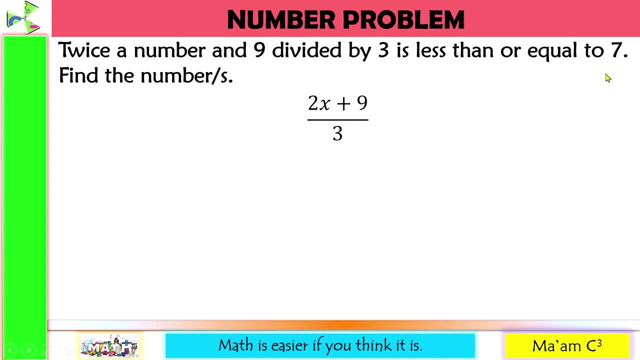 over 3 is less than or equal to 7.. Less than or equal to 7.. To solve for x here we have to eliminate this denominator here. To do that, we are going to multiply both sides by 3.. So 3 here. 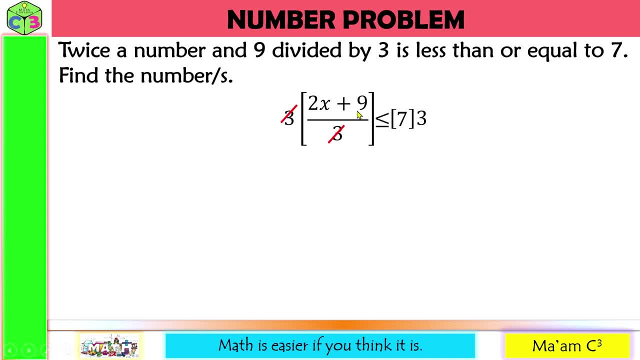 will cancel out. We'll have here 2x plus 9.. On this side, 7 times 3 is 21.. Let us move 9 to the other side. It will become negative. 21 minus 9 is 12.. 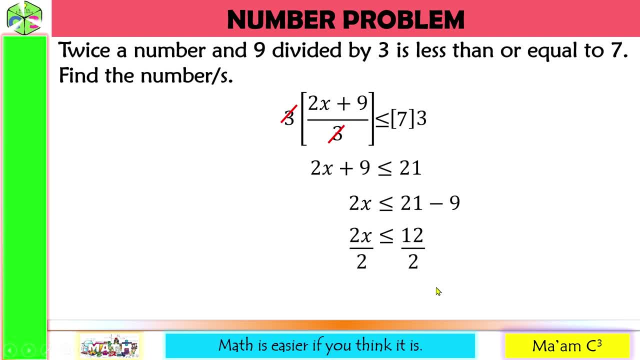 To solve for x, let us divide both sides by 2.. 2 here will cancel out, And 12 divided by 2 is 6.. Let us check. Let us say our x is equal to 6.. So if this is 6, 2 times 6 is 12.. 12 plus 9 is 21.. 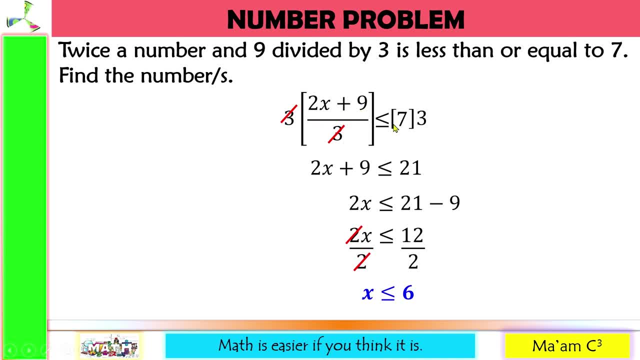 And 21 divided by 9 is 6.. So if this is 6, 2 times 6 is 12.. 12 plus 9 is 21.. And 21 divided by 3 is equal to 7.. Correct Now, what if our x is equal to 3? 2 times 3 is 6.. 6 plus 9 is 15.. 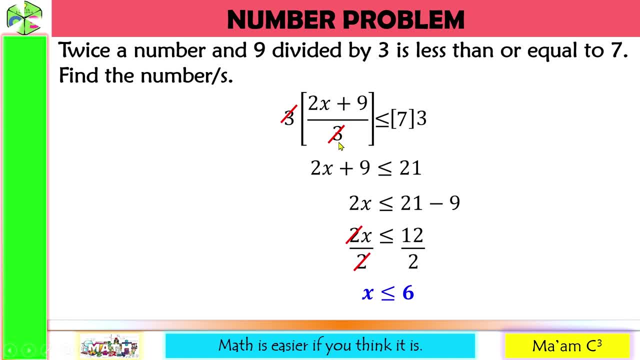 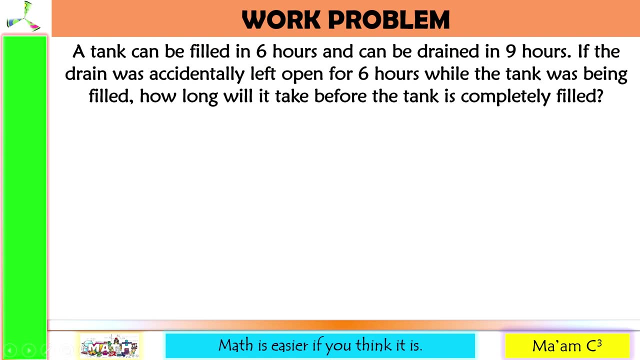 15 divided by 3 is equal to 5. And 5 is less than 7.. Also correct Again, the numbers are: x is less than or equal to 6.. Let us have work problem. A tank can be filled in 6 hours. 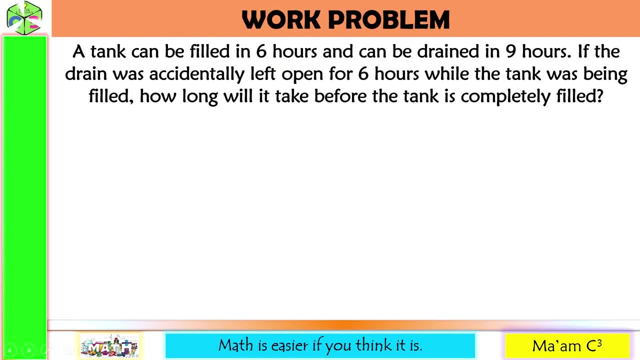 And can be drained in 9 hours. If the drain was accidentally left open for 6 hours while the tank was being filled, how long will it take before the tank is completely filled For work problem? you have to understand that if the work is done, then that is equal to 1.. Now let's have a table. 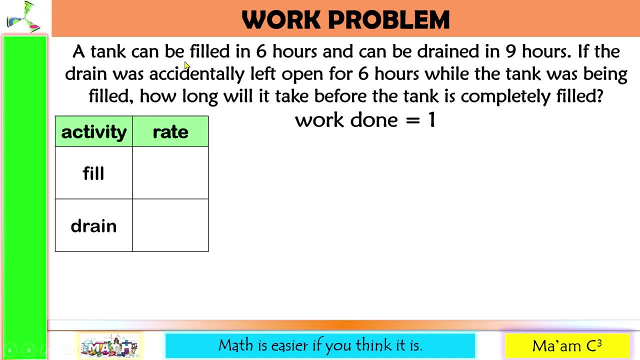 for this. For the fill, a tank can be filled in 6 hours, So meaning the rate is 1 over 6. It means after 1 hour the tank is 1 sixth filled. The drain it can be drained in 9 hours. So the rate. 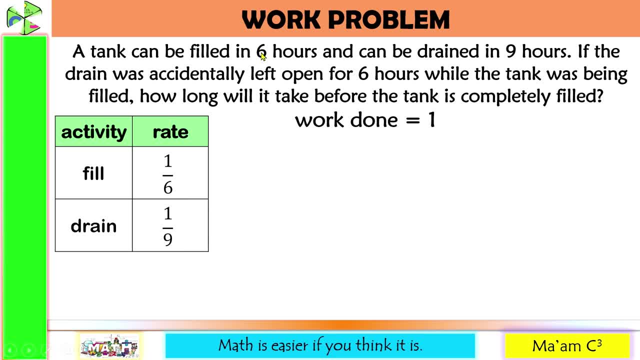 is 1 over 9.. While filling the tank, the drain was accidentally left open for 6 hours. So we are asked now: how long will it take before the tank is completely filled? So the rate for filling is 1 over 6.. We are asked how long will it take? So that would be x, As the tank is being filled. 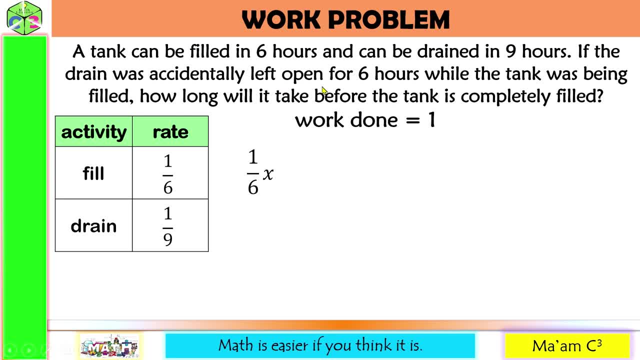 the drain was accidentally left open, So the rate for drain is 1 over 9.. We are going to subtract that For how many hours that the drain was left open- For 6 hours, So we are going to multiply the rate of drain by 6.. How long will it take before the tank is completely filled, Meaning the work? 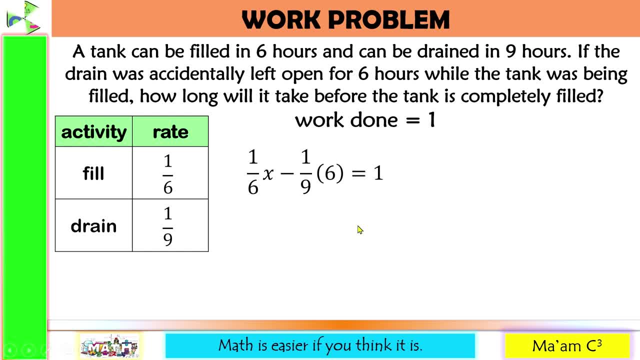 is done, So this is equal to 1.. First step here is to solve for the LCD. The LCD is filled with 6 and 9 is 18.. 18 divided by 6 is 3 times 1 is 3 times x is 3x. 18 divided by 9 is 2 times 1 is. 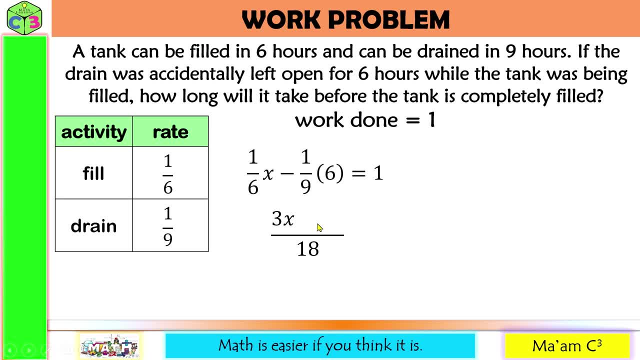 still. 2 times 6 is 12 minus 12.. Copy equals 1. To eliminate this 18 here, we're going to multiply both sides by 18.. So this 18 here will cancel out. We'll only have 3x minus 12 on the left side. 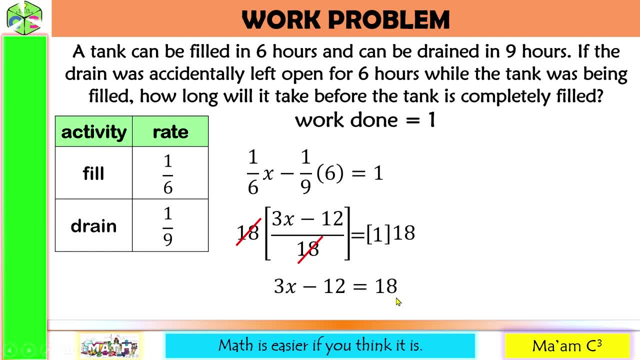 And 1 times 18, 18 on the right side. Let us move negative 12 to the other side, It will become positive. 18 plus 12 is equal to 30.. To solve for x, let us divide both sides by 3.. This 3 here will: 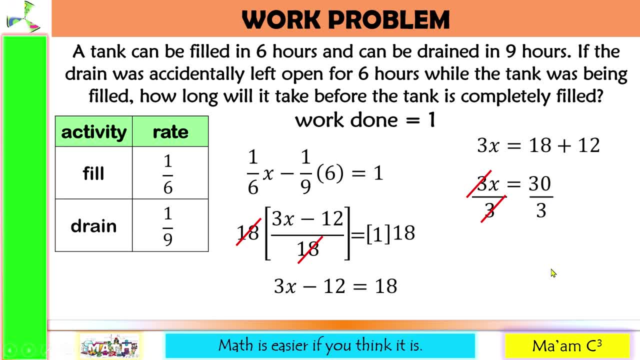 cancel out. 30 divided by 3 is equal to 10.. So this means it would take 10 hours to completely fill the tank. It would have been 6 hours only, But since the drain was accidentally left open for 6 hours, it would take 10 hours to completely. 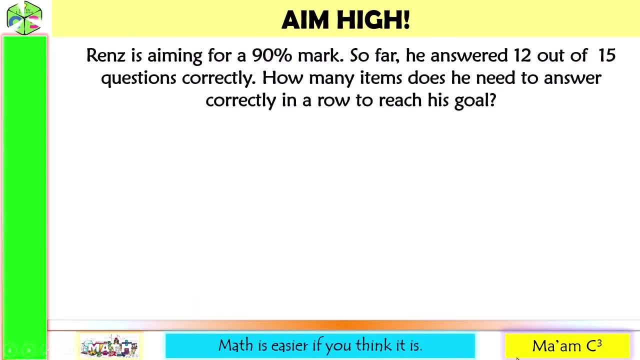 fill the tank. Another one: Renz is aiming for a 90% mark. So far, he answered 12 out of 15 questions correctly. How many items does he need to answer correctly in a row to reach his goal? So far, he answered 12 out of 15 questions correctly, and that is 0.67.. 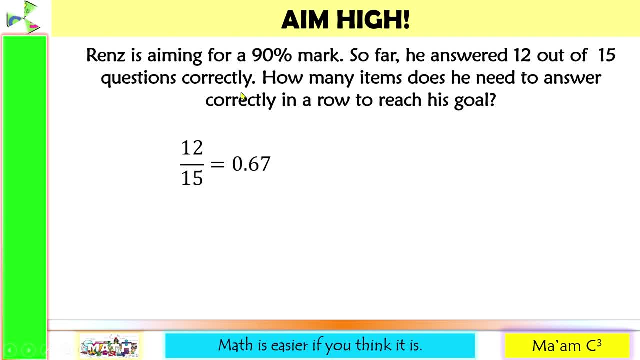 We are asked how many items does he need to answer correctly in a row? So from 12 over 15, we are going to add the number of items that he needs to answer correctly in a row. So that would be plus x. Whatever is the number of items you add here will also be added in the total number. 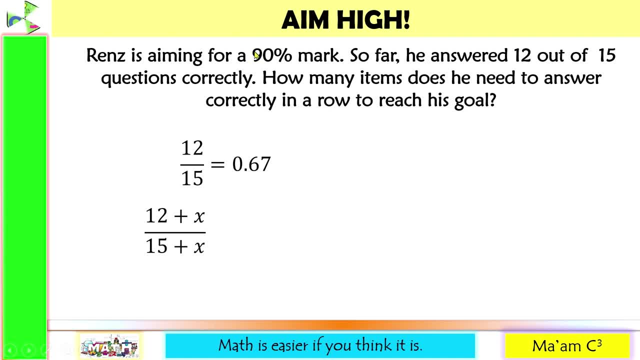 of items, But this time he wants his mark to be 90%, So equal to 0.90.. To eliminate this 15 plus x here, let us multiply both sides by 15 plus x, So this 15 plus x will. 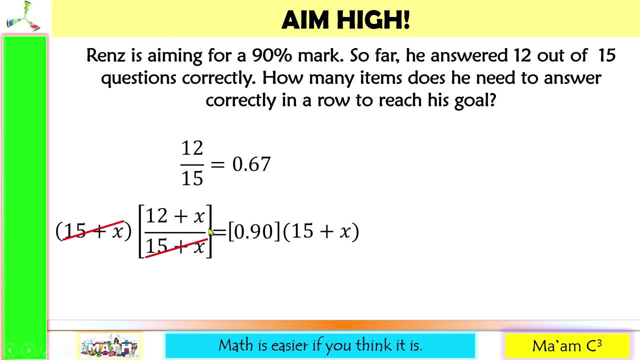 cancel out. On the left side, we'll only have 12 plus x. Now for the right side, we have 0.9 times 15 plus x. Let us copy: 12 plus x. 0.90 times 15 is equal to 13.5.. 0.90 times x is 0.90.. 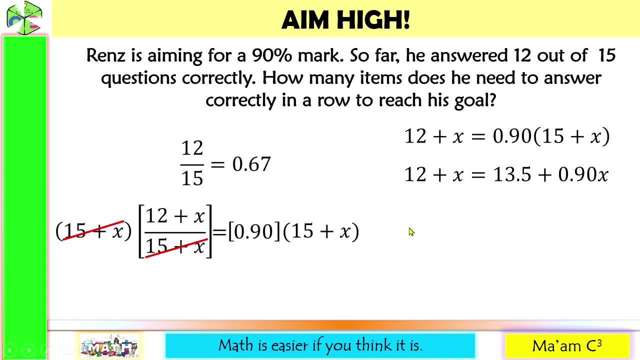 So we have 0.90 times x. Let us copy 12 plus x. 0.90 times 15 is equal to 13.5.. 0.90 times x is 0.90. x- Let us combine like terms. Let us copy x here. Let us move 0.90 x on this side, So this will be: 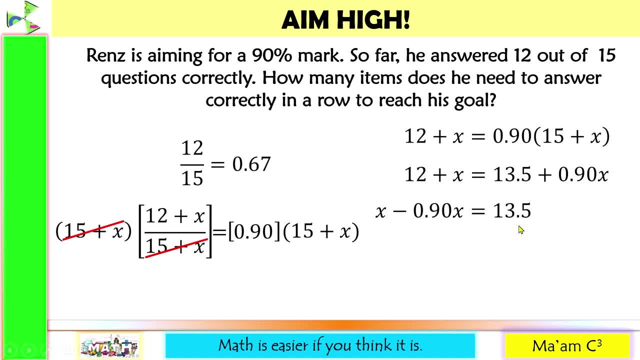 minus 0.90 x. Let us copy 13.5.. Let us move 12 together with this constant, It will become minus 12.. The numerical coefficient of x here is 1.. So 1 minus 0.90 x is 0.10 x or 0.1 x. 13.5 minus 12. 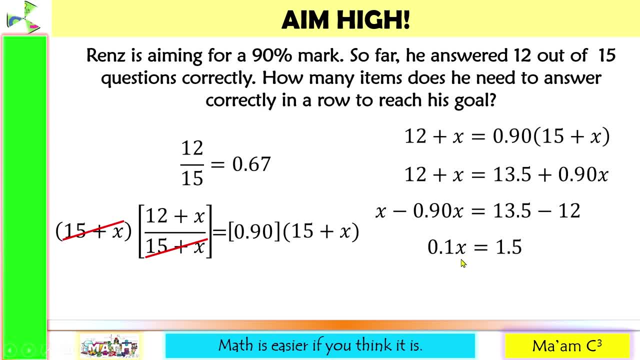 is equal to 1.5.. To solve for x, let us divide both sides by 0.1.. This 0.1 here will cancel out. 1.5 divided by 0.1 is equal to 15.. So this: 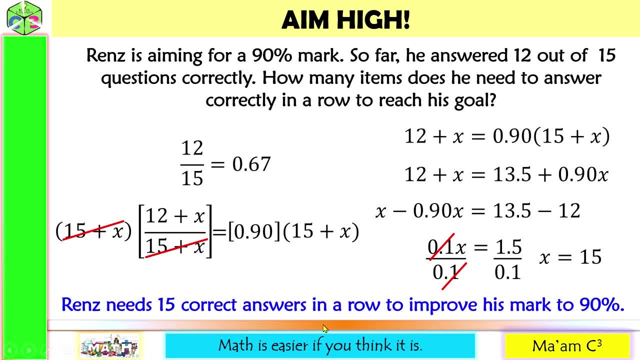 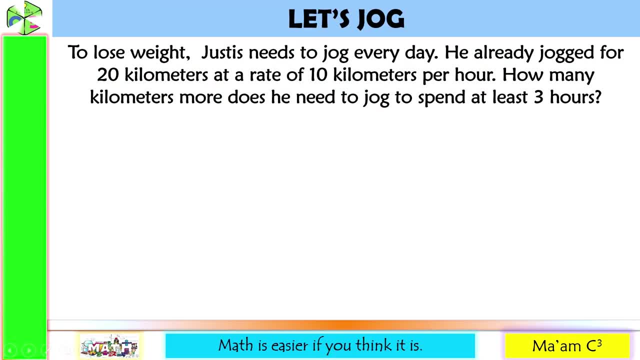 means that means Renz needs 15 correct answers in a row to improve his mark to 90 percent. Let's jog To lose weight. Justice needs to jog every day. He already jogged for 20 kilometers at a rate of 10 kilometers. 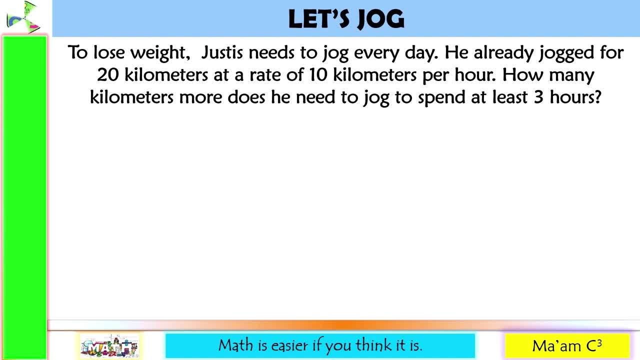 per hour? How many kilometers more does he need to jog to spend at least three hours? Let us have again our magic triangle. This time we have D for distance, R for rate and T for time. If we want to solve for distance, let us cover D, and D is equal to rate times T. If we want to solve for the rate, 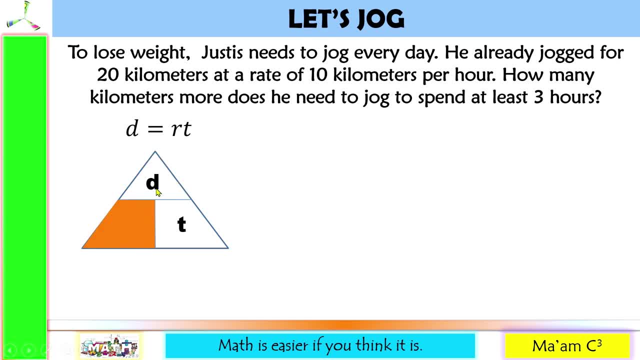 let us cover R, and R is equal to D divided by T. And if we want to solve for the time, let us cover T, and T is equal to D divided by R. Now it says here to spend at least three hours. At least three hours meaning you cannot go below. 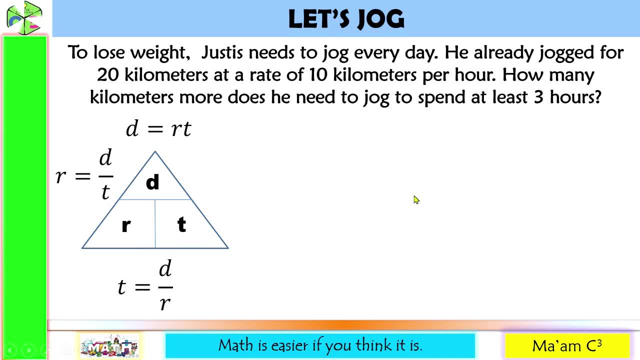 three hours, So it could be greater than or equal to three. This three here is time. So we're going to use this formula: Distance divided by the rate. The distance is already given 20 kilometers and the rate is also given 10 kilometers. 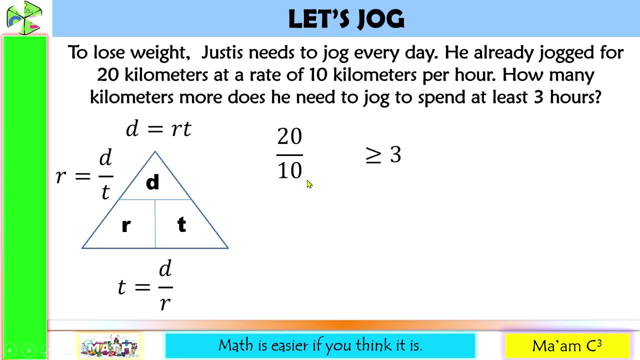 So it's 10 kilometers per hour, So divided by 10.. We are asked: how many kilometers more does he need to jog? So we're going to add additional distance. Distance is X and the rate is constant, which is 10.. So plus X over 10.. To solve for X, let us first eliminate this 10 here. Let us multiply both sides. 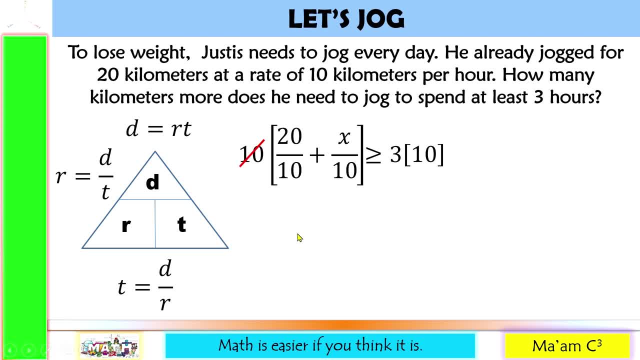 by 10.. So 10 here will cancel out, leaving us 20.. This time this 10 will cancel out, leaving us X. Three times 10 is 30. Let us move 20 to the other side, It will become minus 20.. And 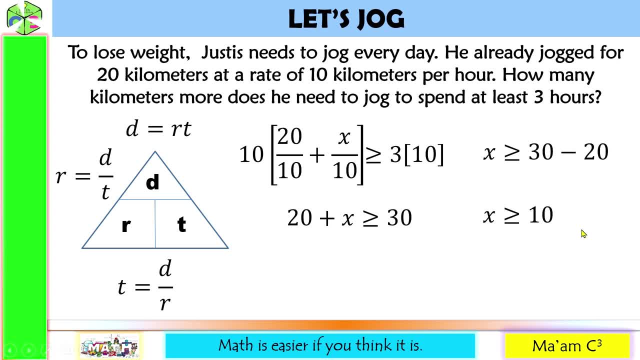 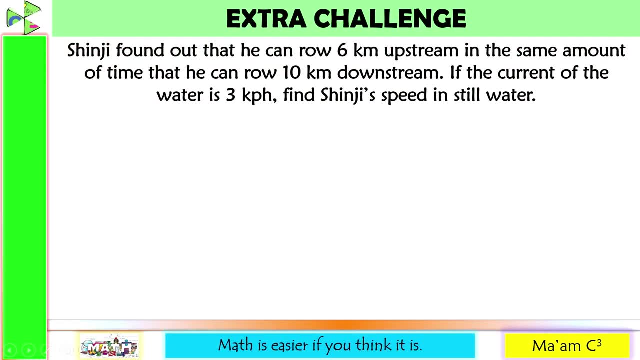 30 minus 20 is equal to 10.. So this means Justice needs to jog greater than or equal to 10 kilometers more to spend at least three hours of jogging. Let us do extra challenge. Shinji found out that he can row six kilometers more than or equal to 10 kilometers more than the distance he was given. 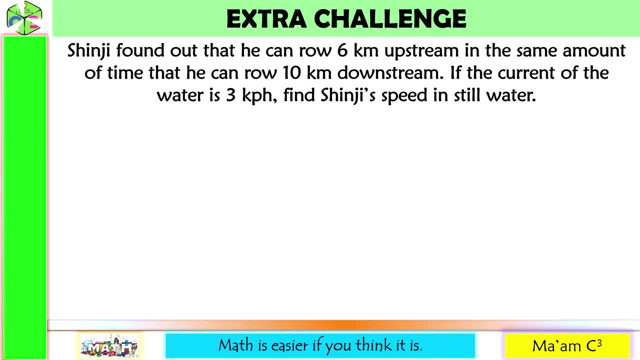 upstream in the same amount of time that he can row 10 kilometers downstream. If the current of the water is 3 kilometers per hour, find Shinji's speed in still water. For this kind of problem we have a general formula for the rate and that is equal to the speed of the vehicle in still water. 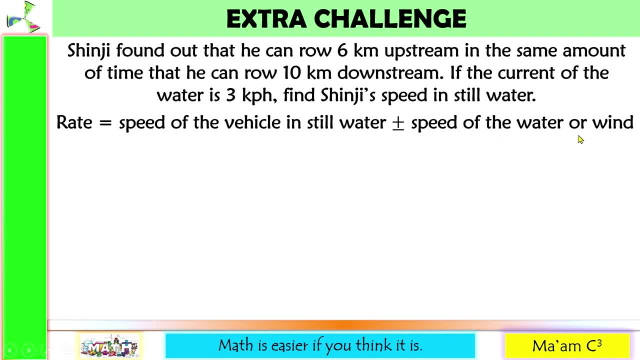 plus and minus the speed of the water or the wind. Let us let X be the speed in still water and let C be the speed of the current. You are actually dealing with three speeds in this problem: The speed in still water, the speed if you are going against the current, and the speed. 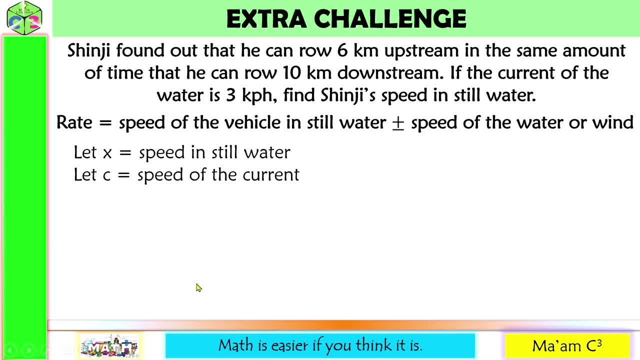 if you are going with the current. So let's have a table: Upstream and downstream, distance, rate and time. the distance for upstream is given and that is six kilometers. for downstream, that is 10 kilometers. now for the rate. again, that would be the speed of the vehicle. 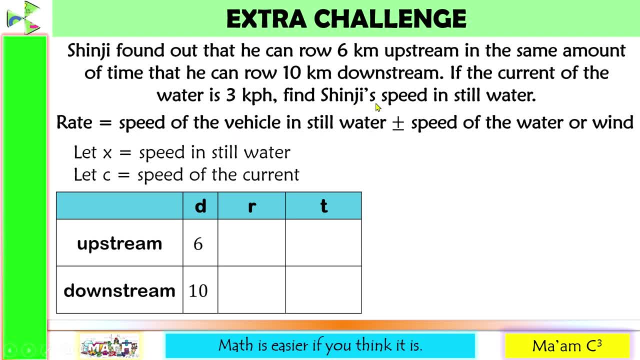 in still water and that is what we are asked in this problem. so this will be x plus or minus the speed of the water or wind. the speed of the water or the current of the water is three kilometers per hour. if you are going upstream, you are going against the current. so this is minus three if you 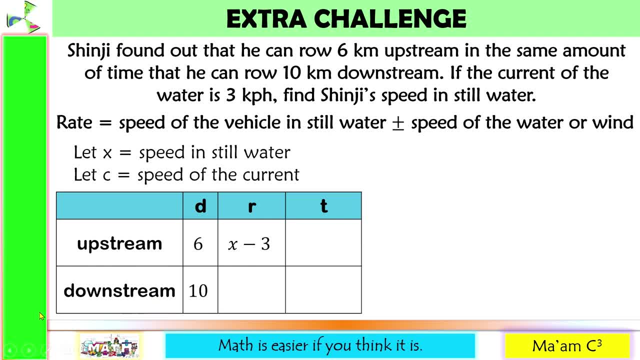 are going downstream, you are going with the flow of the current, so this will be x plus three. now for the time. let us recall our triangle. if we want t, let's go over t, and that would be equal to distance divided by r. we already have the distance. 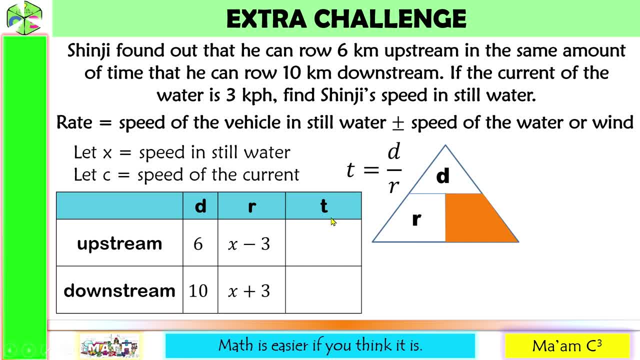 we already have the rate. so our t is d divided by r, so six divided by x minus three. for downstream it would be 10 divided by x plus three. it says here same amount of time. so the time is spent going upstream is equal to the time is spent going downstream. let's do a little shortcut here. let. 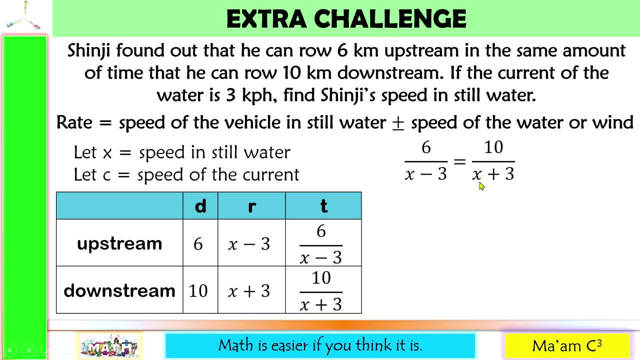 us do cross multiplication: six times x plus three is equal to ten times x minus three. six times x is six x. six times three is eighteen. ten times x is 10 x. ten times negative three is minus 30.. let us combine like terms. let us find out that the times with one half increased up. let us combine like terms. let us find out that the times with one half increased up. in the end this is stretching up from three to the half, where x is equal to three and we kx is negative three, so x is minus 30, which is negative three as a number. three and yo, we mean there is not going upwards a result for us that we will have to mental Romanian speed. so we can't count what we can do if we want to know this in the next. 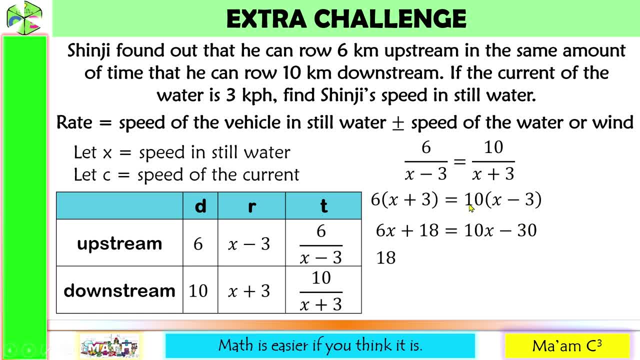 copy 18 here. Let us move negative 30 together with this constant, It will become plus 30.. Let us copy 10x. Let us move 6x to this side, It will become minus 6x. 18 plus 30 is 48.. 10x. 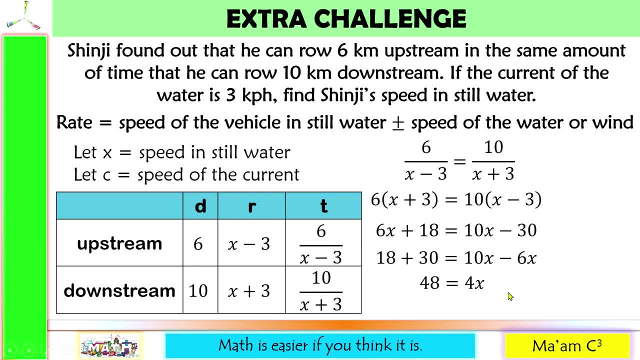 minus 6x is equal to 4x. To solve for x, let us divide both sides by 4.. So this 4 here will cancel out. 48 divided by 4 is equal to 12.. This means Shinji's speed in still water is 12. 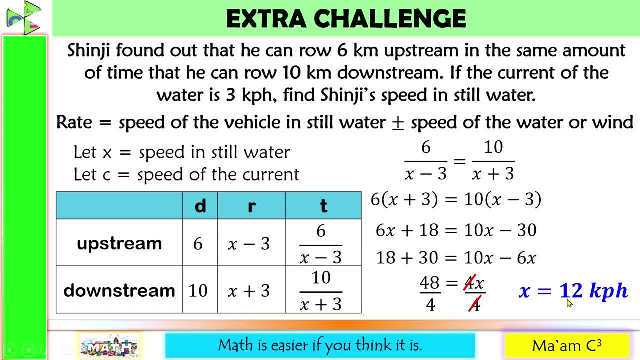 kilometers per hour. Let us check if this is 12.. So 12 minus 3 is 9.. 6 divided by 9, in lowest term, is two-thirds. If this is 12,, 12 plus 3 is 15.. 10 divided by 15, in lowest term, is also. 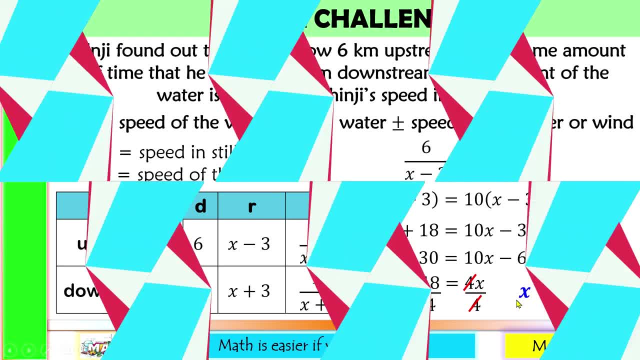 two-thirds. If this is 12,, 12 plus 3 is 15.. 10 divided by 15, in lowest term, is also two-thirds. So this is correct. Now it is time to check your understanding. Pause this video for more time. 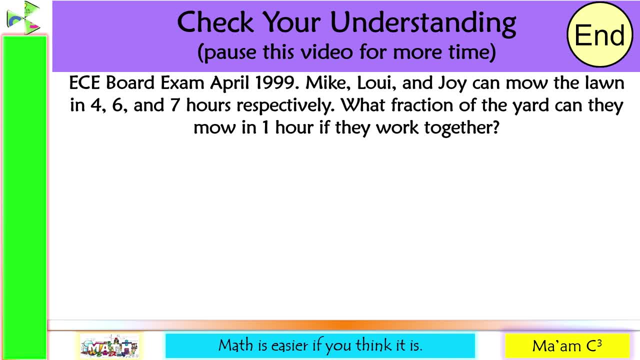 Let us answer. So. this is from ECE board exam of April 1999.. Mike, Louie and Joy can mow the lawn in 4, 6, and 7 hours Respectively. what fraction of the yard can they mow in 1 hour if they work together? 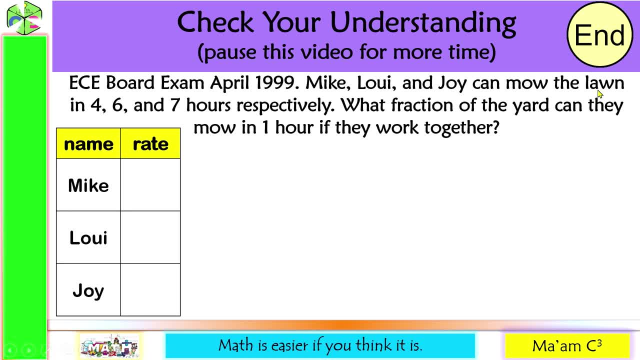 Let us have our table. Mike can mow the lawn in 4 hours, So his rate is 1 over 4.. Louie can mow the lawn in 6 hours, So his rate is 1 over 6.. And Joy can mow the lawn in 7 hours. 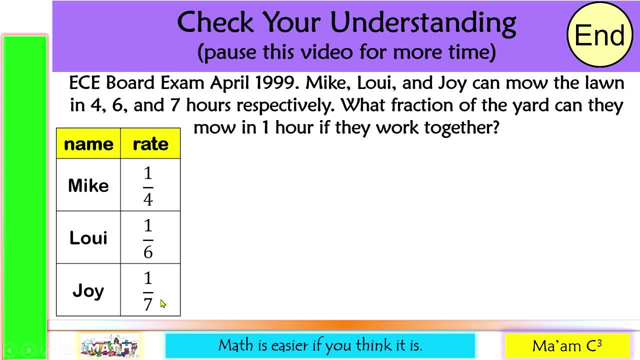 It means her rate is 1 over 7.. What fraction of the yard can they mow in 1 hour if they work together? Work together? So meaning we are going to add their rates. So we have 1 fourth plus 1 sixth plus 1 over 7.. 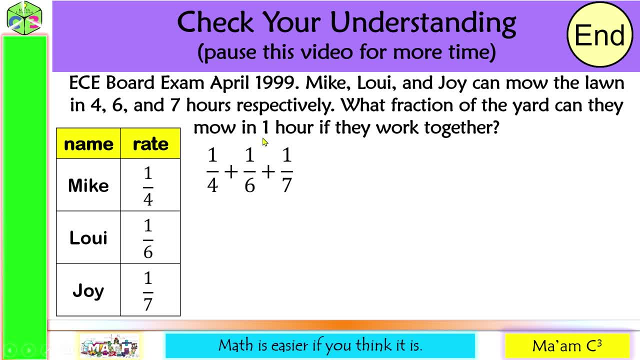 Now for how long they work together? For 1 hour. So we are going to multiply their rates by 1 hour. So what fraction of the yard has been finished after working together for 1 hour? This is equal to X. We are asked: what fraction have been finished after working together for 1 hour? 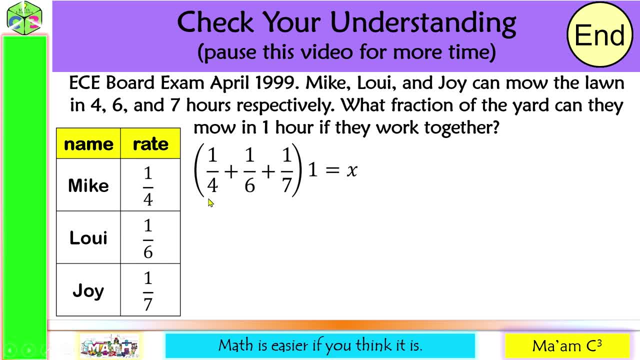 The next thing to do here is to determine the LCD. Let's have a quick review. in determining the least common denominator, All you have to do is to determine the prime factors of the denominators. Let us start with 4.. 4 is equal to 2 times 1.. 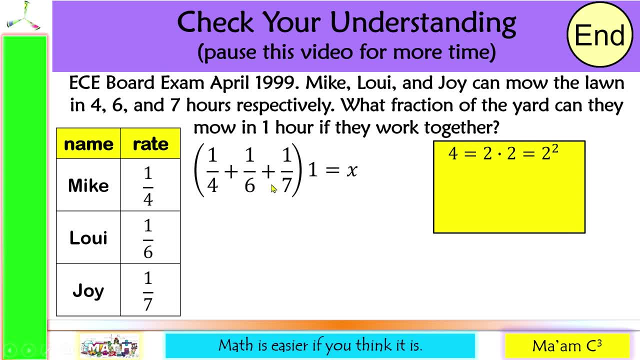 4 is equal to 2 times 1.. 4 is equal to 2 times 2, or 2 squared, 6 is equal to 2 times 3.. 7 is equal to 7 times 1.. Afterwards you are going to choose the prime factors having the highest exponent. 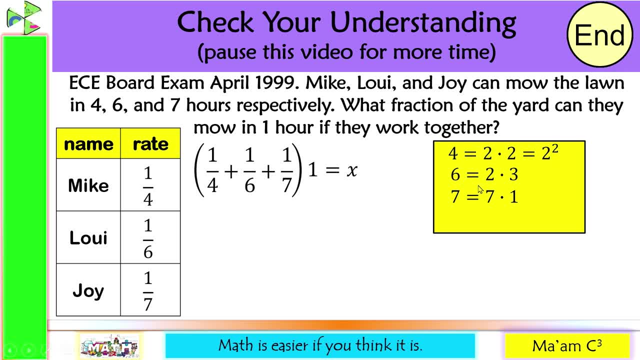 Let us have 2.. So here we have 2 squared. Here we have 2 to the first, power 2 is greater than 1.. So we are going to choose 2 squared. Now for 3, we only have 1, 3.. So we are going to choose this. 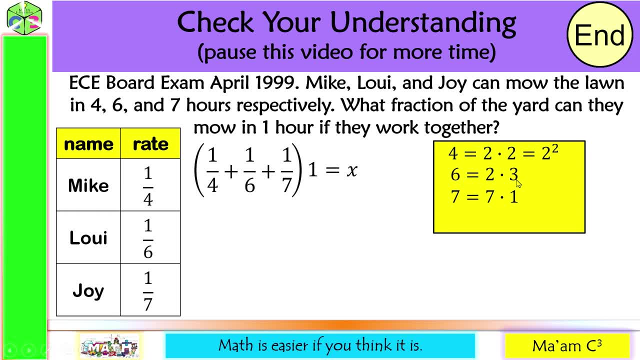 Same thing with 7.. There are no other 7 here, So we are going to choose 7.. 1, it doesn't matter, It will not affect our LCD. So again, we choose 2 squared 3 and 7..